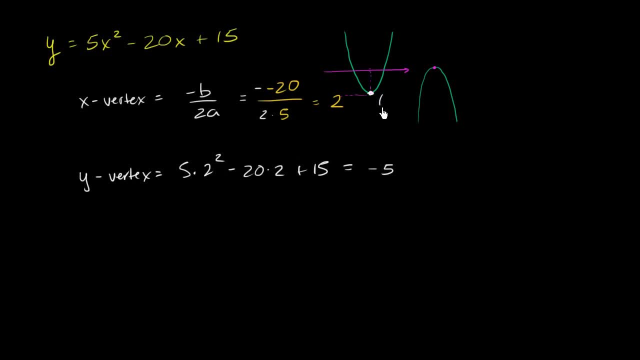 So just like that, we're able to figure out the coordinate. This coordinate right over here is the point 2 comma negative 5.. Now it's not so satisfying just to plug and chug a formula like this And we'll see where this comes from. 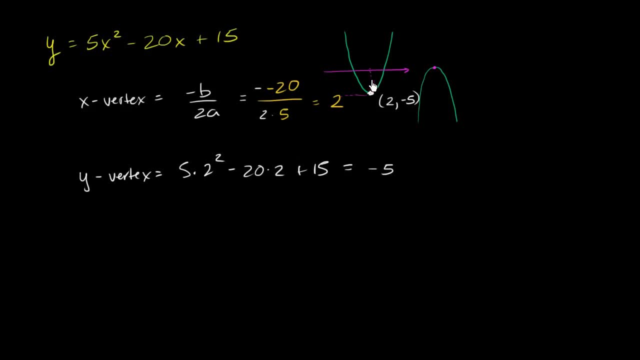 when you look at the quadratic formula, This is kind of the first term. It's the x value that's halfway in between the roots. So that's one way to think about it, But another way to think about it and another way to do it, and this probably 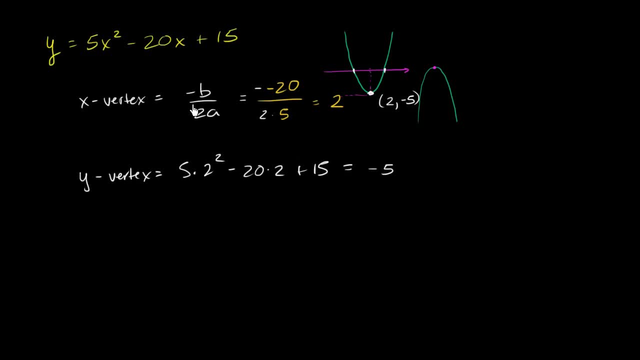 will be of more lasting help for you in your life, because you might forget this formula is to really just try to remanipulate this equation so you can spot its minimum point, And we're going to do that by completing the square. 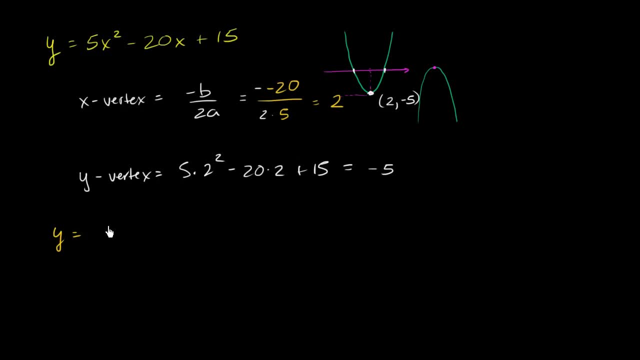 So let me rewrite that. So we have: y is equal to, and I'll write it as, and what I'll do is, out of these first two terms, I'll factor out a 5, because I'm going to complete a square here. 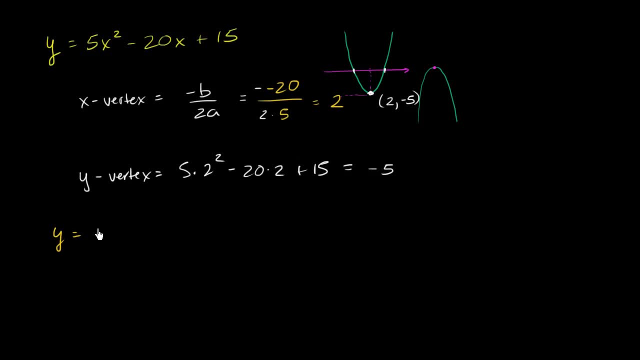 And I'm going to leave this 15 out to the right because I'm going to have to manipulate that as well. So I'll write that as 5 times x squared minus 4x, And then I have this 15 out here. 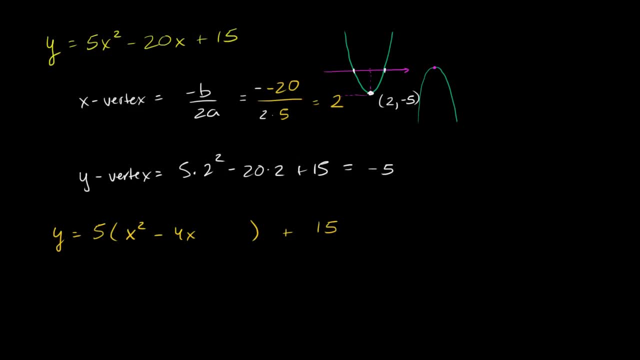 And I want to write this as a perfect square, And we just have to remind ourselves that if I have x plus a squared, that's going to be x squared plus 2ax plus a squared. So if I want to turn something that looks like this: 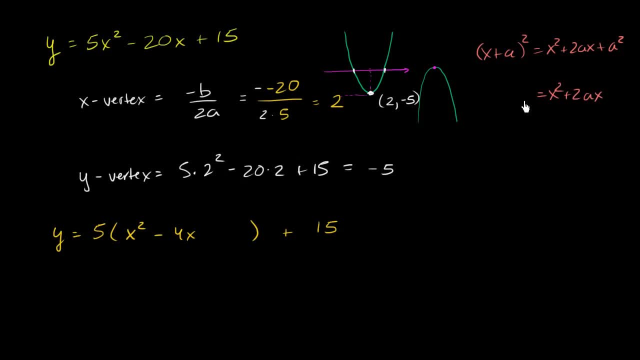 if I want to turn something like this 2ax into a perfect square, I just have to take half of this coefficient And square it and add it right over here in order to make it look like that. So I'm going to do that right over here. 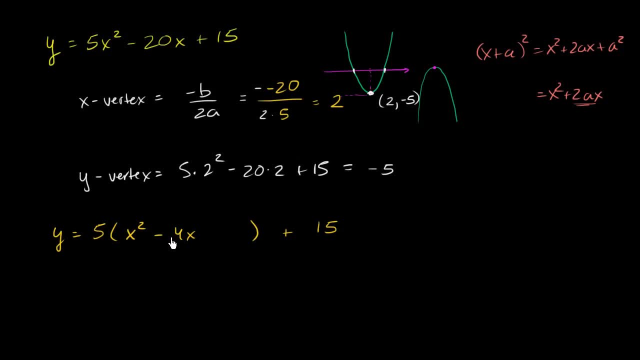 So if I take half of negative 4, that's negative 2. If I square it, that is going to be positive 4.. I have to be very careful here. I can't just willy nilly add a positive 4 here. 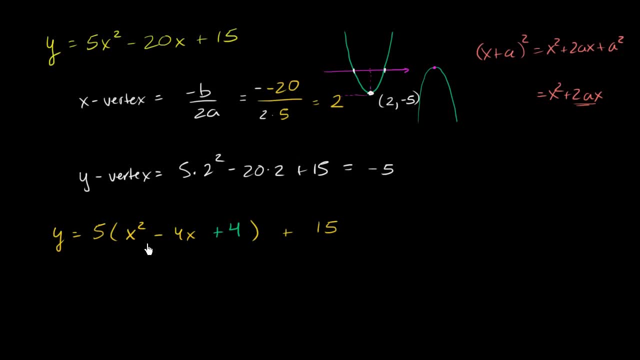 I have an equality here. If they were equal before adding the 4, then they're not going to be equal after adding the 4.. So I have to do proper accounting here. I either have to add 4 to both sides or actually. 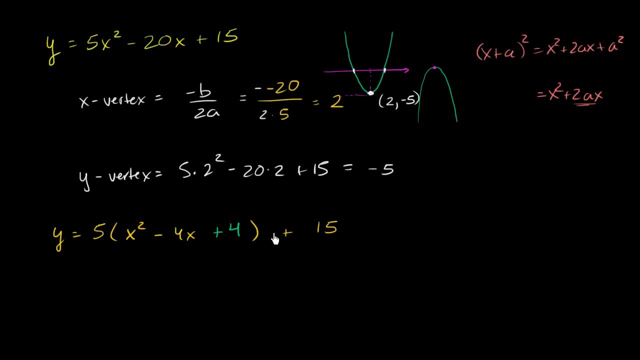 be careful. I have to add the same amount to both sides just like that, or subtract the same amount again. Now, the reason why I was careful there is: I didn't just add 4 to the right-hand side of the equation. 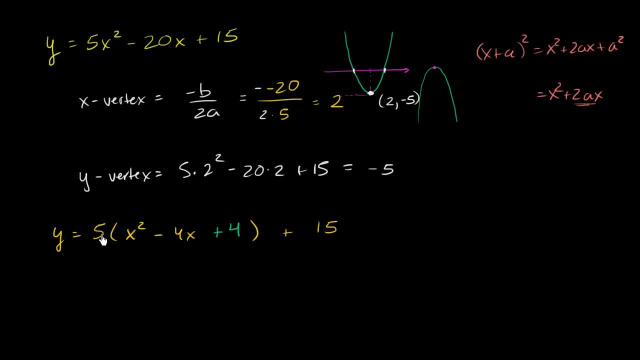 Remember, the 4 is getting multiplied by 5.. I have added 20 to the right-hand side of the equation. So if I want to make this balance out, if I want the equality to still be true, I either have to now add 20 to y. 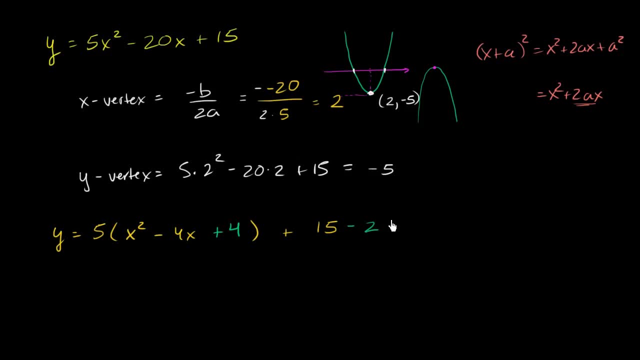 or I have to subtract 20 from the right-hand side. So I'll do that. I'll subtract 20 from the right-hand side. So I added 5 times 4.. If you were to distribute this, you'll see that. 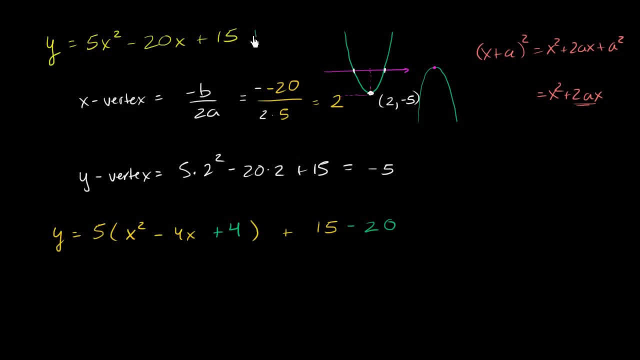 I could have literally up here said: hey, I'm adding 20, and I'm subtracting 20.. This is the exact same thing that I did over here. If you distribute the 5,, it becomes 5x squared minus 20x. 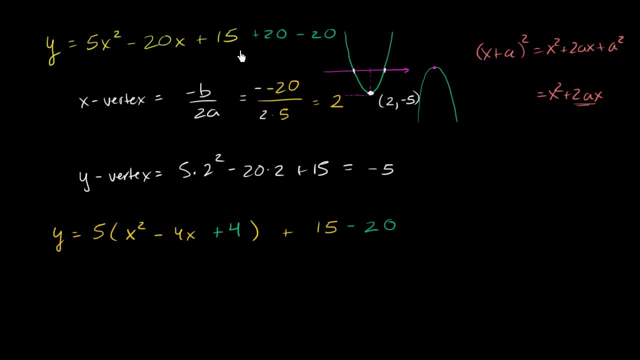 plus 20, plus 15 minus 20, exactly what's up here. The whole point of this is that now I can write this in an interesting way. I could write this as: y is equal to 5 times x minus 2.. squared, and then 15 minus 20 is minus 5.. 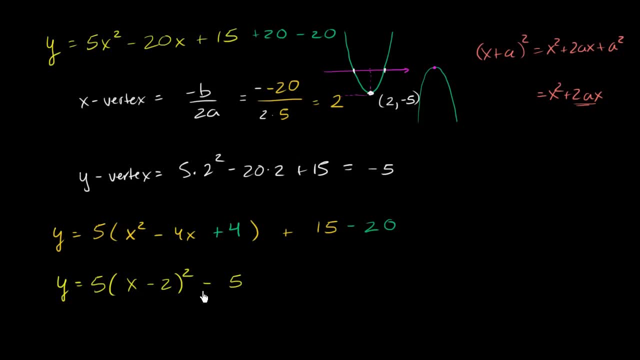 So the whole point of this is now to be able to inspect this. When does this equation hit a minimum value? Well, we know that this term right over here is always going to be non-negative, or we could say it's always going to be greater than or equal to 0..